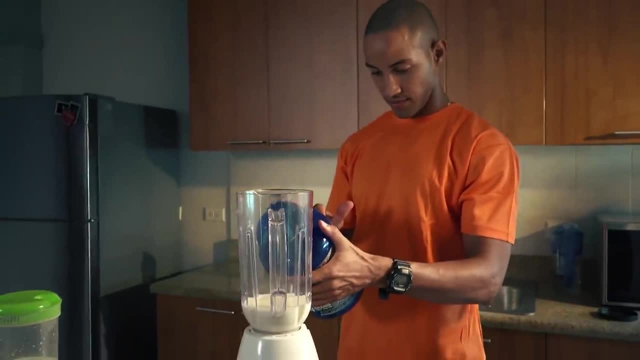 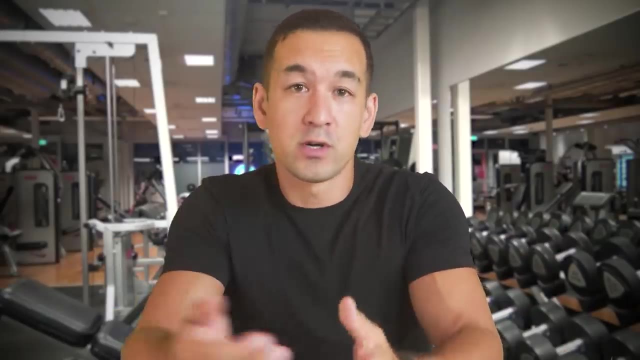 which I'll explain in a second. But maybe your protein powder lists 25 grams of protein per scoop on the label, when in reality it's only 15 grams of protein and then 10 grams of maybe one or two cheap, low quality amino acids that aren't going to have any added muscle building effect. 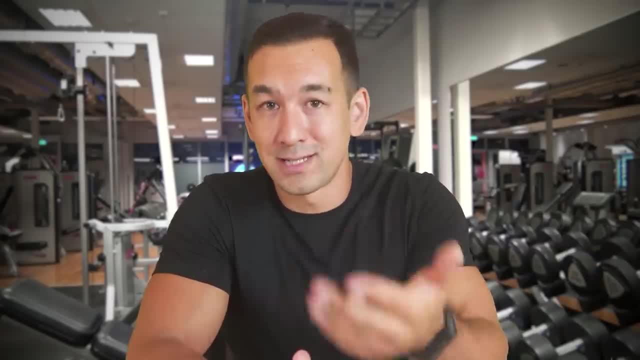 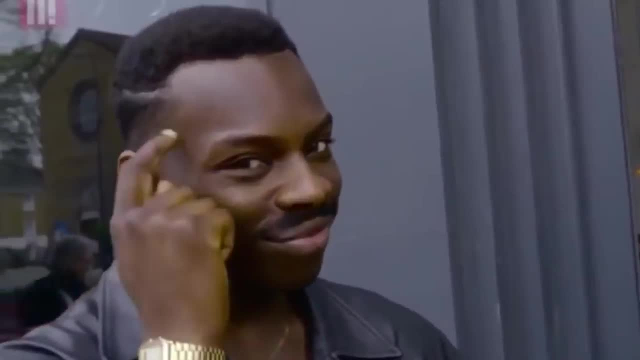 So they make more profit. on each tub you get a lower quality, less effective product. Now, fortunately, amino spiking isn't as common as it was a few years ago, because more and more consumers have caught onto this. but there are still quite a few protein powders out. 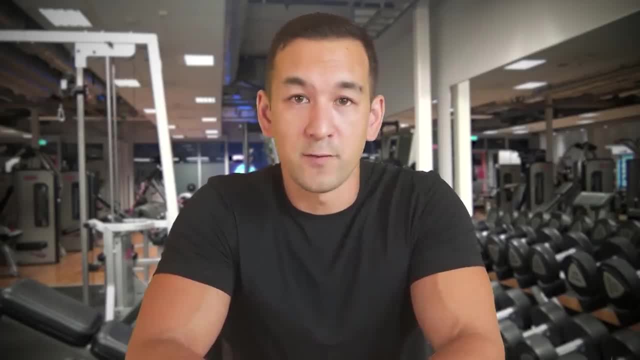 there that are still doing this, And so it is something that you need to be aware of. So how do you know if your protein powder is amino spiked? Well, it's actually pretty simple. You just need to look at the ingredient label, not the amino acid profile. A lot of people get 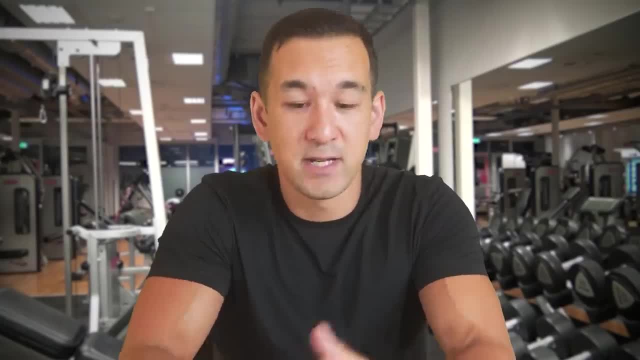 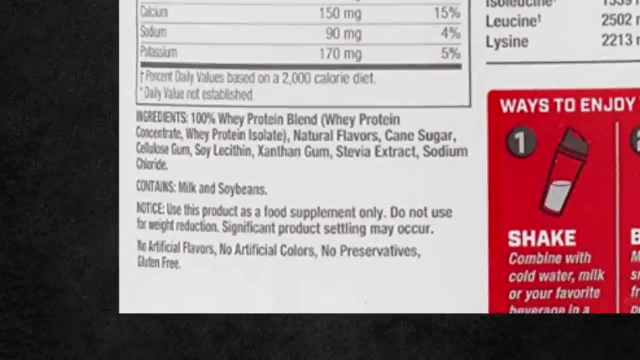 confused on this. Every protein powder contains amino acids because they're the building blocks of protein. So having an amino acid profile listed is fine, but what you want to specifically look at here is the ingredient list, which is usually underneath the supplement facts. So what you want 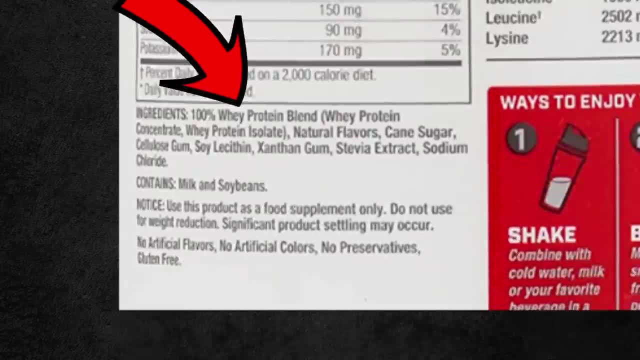 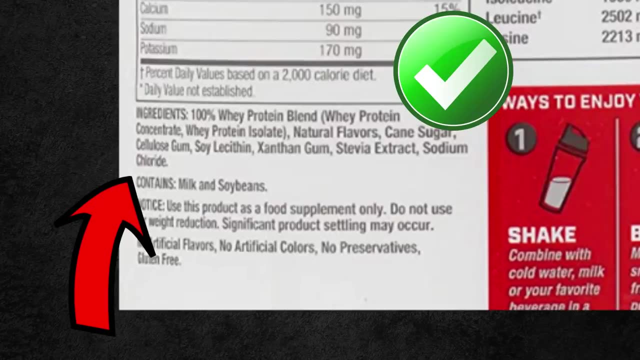 to see is simply the type of protein that's being used as the first ingredient, and then whatever additional flavors and sweeteners and binding agents are being used after that. But what you don't want to see here in this list are singular amino acids. When it comes to amino spiking, 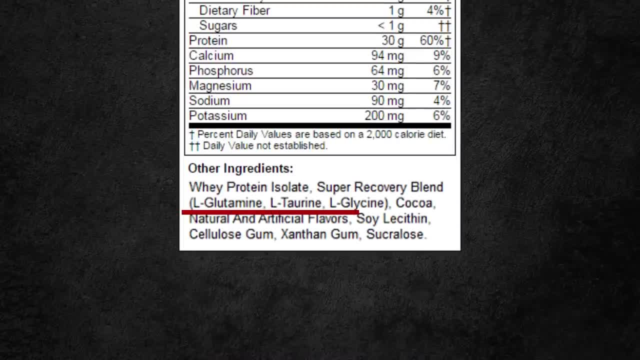 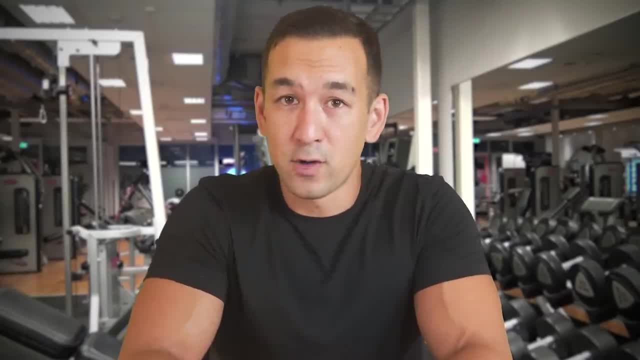 you might see L-glutamine listed, L-taurine, L-glycine- branch chain amino acids are sometimes used because they're actually cheaper gram for gram than protein is. And then another one to look for, and this one might surprise you, because it's something that most people are totally unaware of. 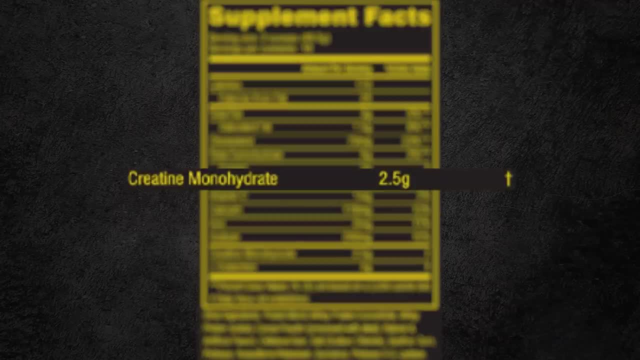 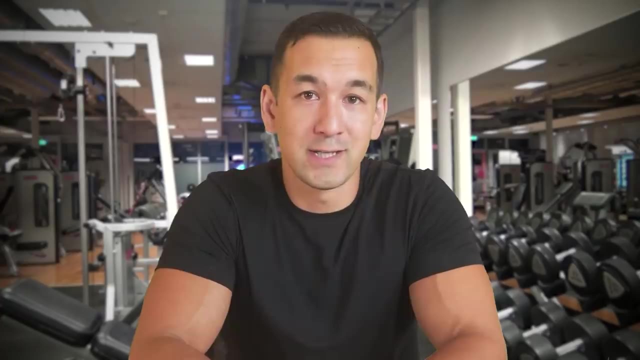 but that is creatine. Oftentimes people will see creatine listed in their protein powder and then they'll think, oh, this is great, What an awesome product. I'm getting 25 grams of protein per scoop and my five daily grams of creatine as well. What an excellent company. They truly care. 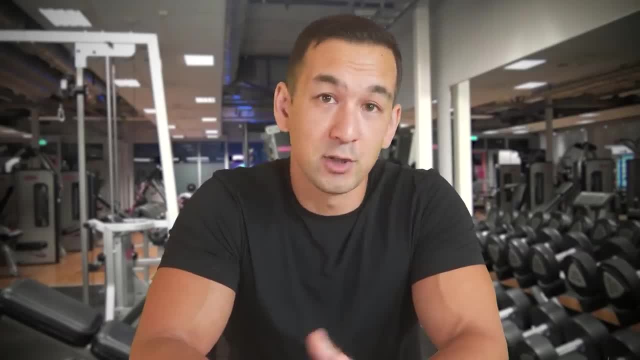 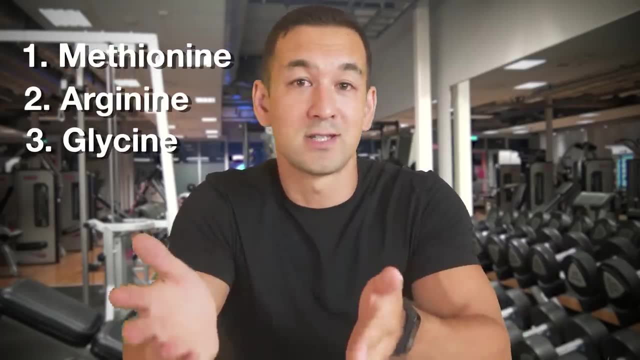 about creating premium quality products. No, actually you just got played, And that's because creatine is actually a combination of three amino acids- methionine, arginine and glycine- And so, even though it's not protein, it's still a. 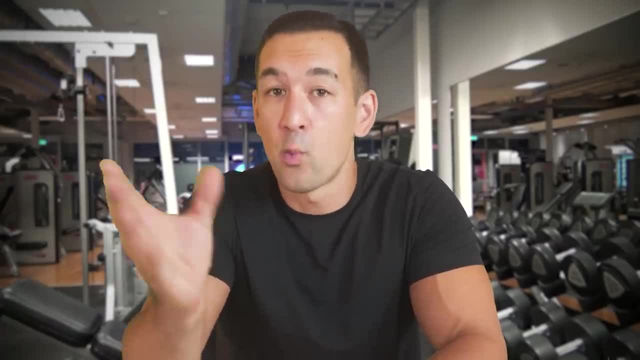 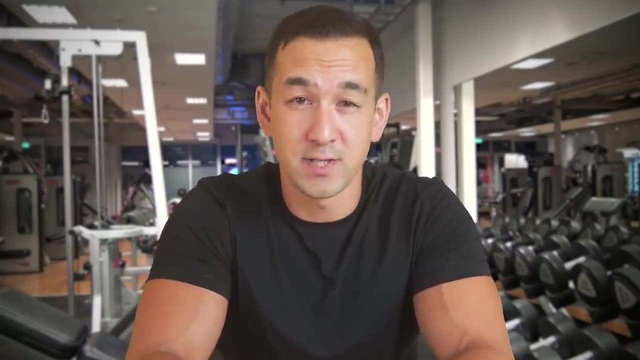 nitrogen containing compound, And so it's actually going to register as protein when that powder gets tested. And not only that, but some tests have actually shown that creatine can register as high as 140% protein. So if the powder has, say, five grams of creatine in it, 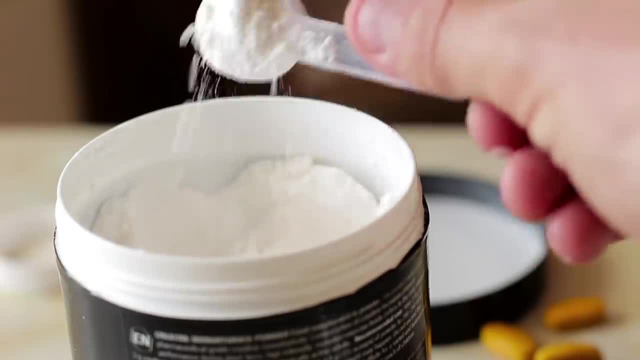 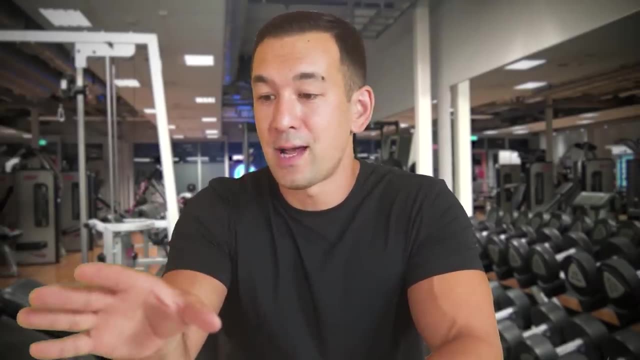 that could be accounting for up to seven or eight grams of the protein total. And companies do this because, gram for gram, creatine is a lot cheaper compared to protein. And it's not only creatine. the same thing also applies to other nitrogenous compounds as well, like beta, alanine or betaine. 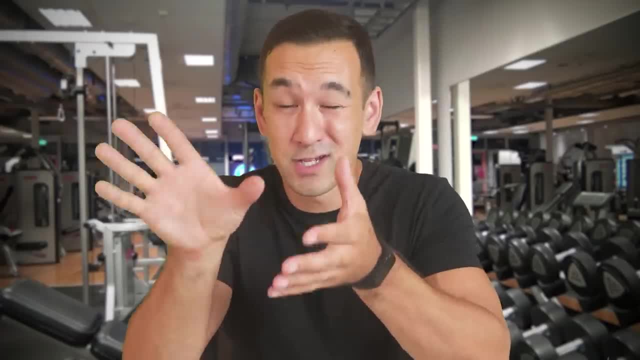 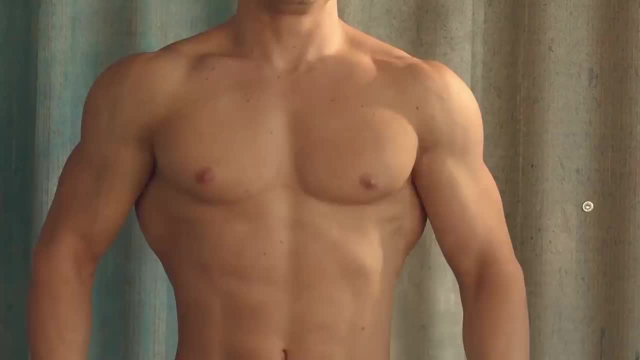 as well. So unless the company specifically states that the protein total is separate from those other ingredients, then there's a very good chance that they're actually using them to artificially inflate the protein total. Now, whether or not amino spiking is actually going to affect your 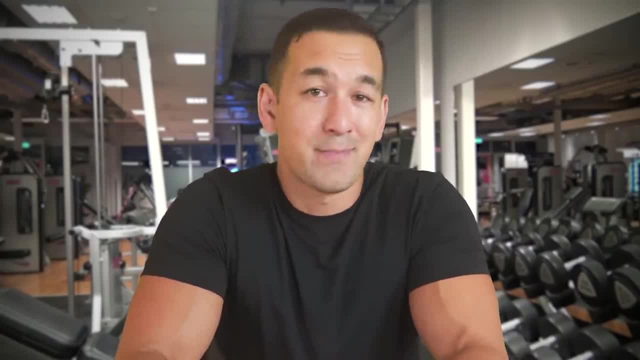 bottom line muscle growth. that will vary from product to product And it just depends how heavily the powder is spiked. You know, if they're just using a few extra grams to shave off a tiny bit of cost per tub, then it's probably not going to matter for you in a practical sense. 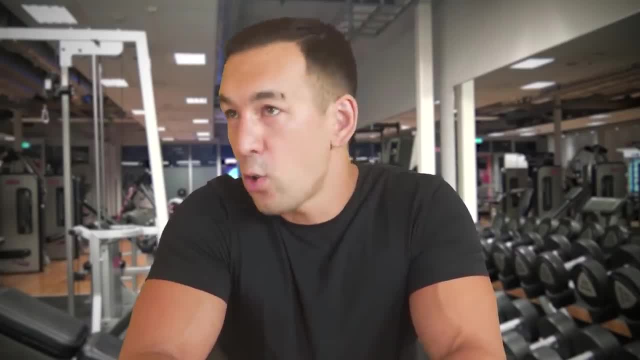 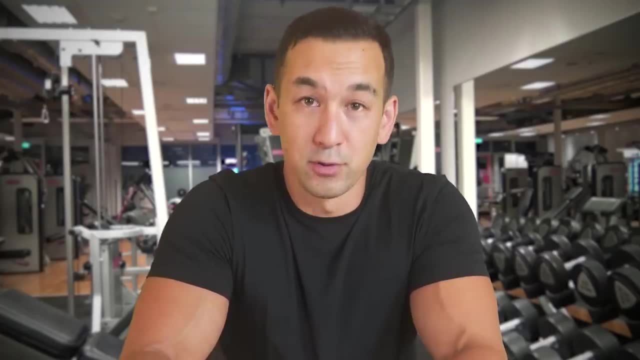 But in any case it's just a flat out misleading tactic. You have no way of knowing how heavily spiked a given powder is, and there's just no reason to give your money to supplement companies that are intentionally bullshitting. you Hit the like button if you agree with that, And moving on. 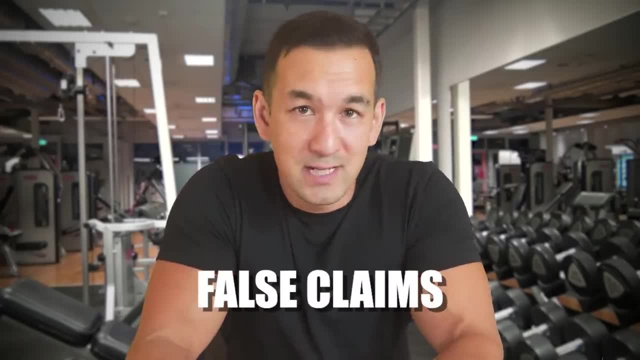 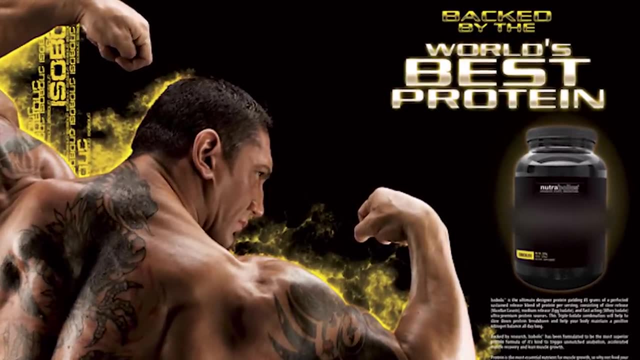 to protein powder. scam number two is just false claims, plain and simple. It's when supplement companies try to portray their protein powder as some kind of high-tech, magical muscle building potion that's going to skyrocket your results in comparison to other protein sources, whether 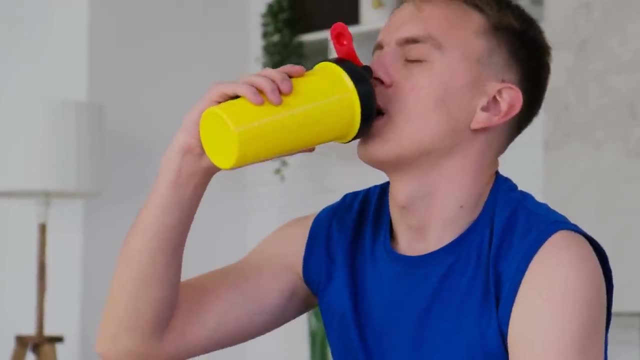 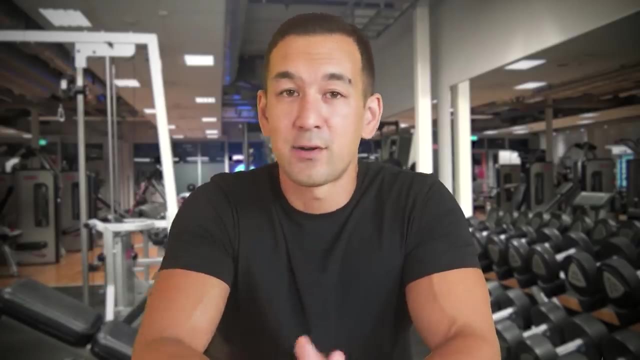 that's a regular solid food protein or a different type of protein powder. Now, yes, on a gram for gram basis. you know it's not going to affect your muscle growth, but it's going to affect your weight. protein, casein, egg white protein, even plant-based powders, if they're formulated. 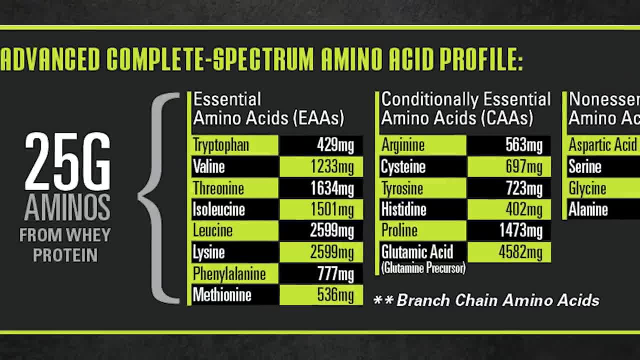 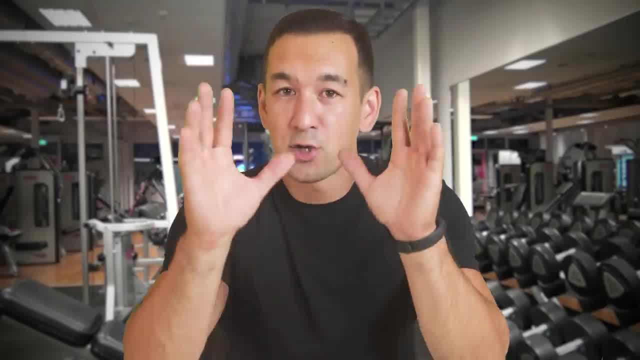 properly. Those are very high quality sources of protein that will have a high bioavailability and a strong amino acid profile, And that's, of course, a good thing. But also keep in mind that, as long as you're consuming enough total protein for the entire day, so around 0.8 grams per pound of body- 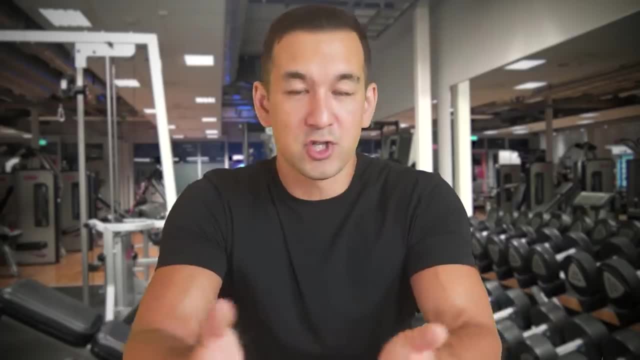 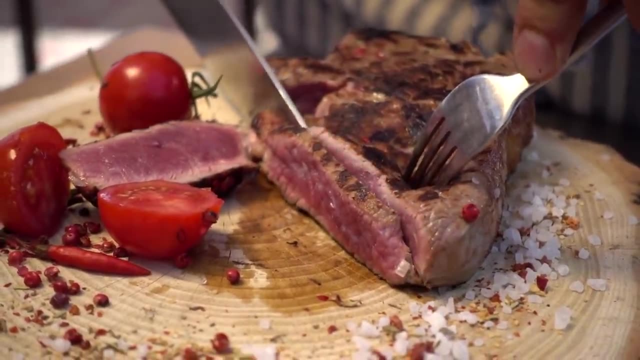 weight, or about 1.8 grams per kilo, and your meals are just generally based around some kind of complete protein source, which most people are going to do by default, even if they don't even lift, you know, chicken, fish, steak, whatever else. If you're doing that, then protein quality. 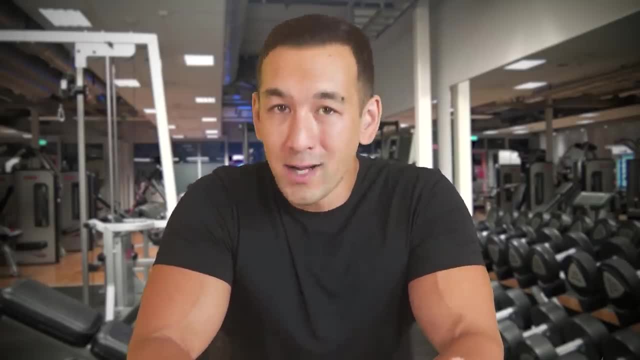 isn't really something you need to obsess over, because with enough total quantity, by the end of the day you'll have gotten all the amino acids that you need to optimize muscle recovery and growth. When it all comes down to it, protein powders really are just optional, You don't? 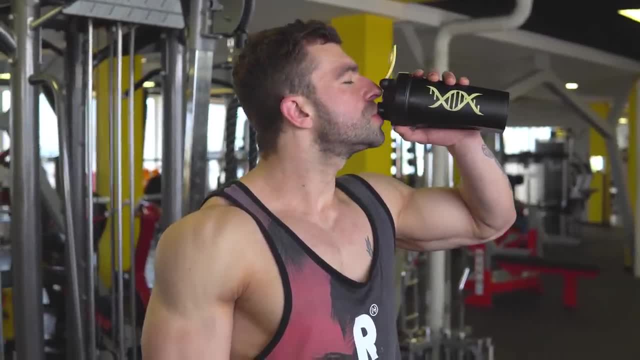 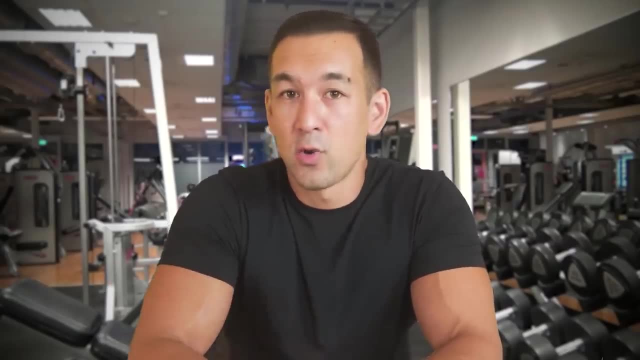 have to use them. You don't have to consume a liquid post-workout shake or a pre-workout shake or take your protein powder before bed. There's no special benefit there, And I even say that as a supplement. I mean it's a supplement, but it's a supplement. It's a supplement, It's a supplement. 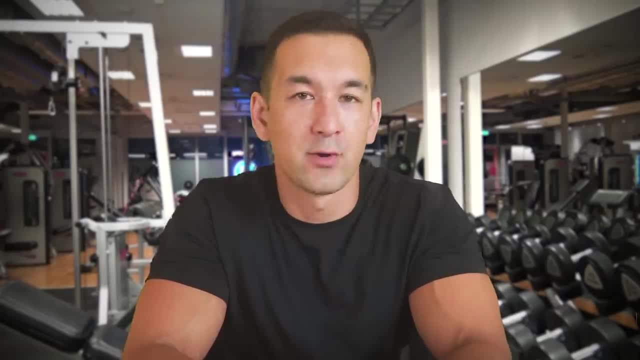 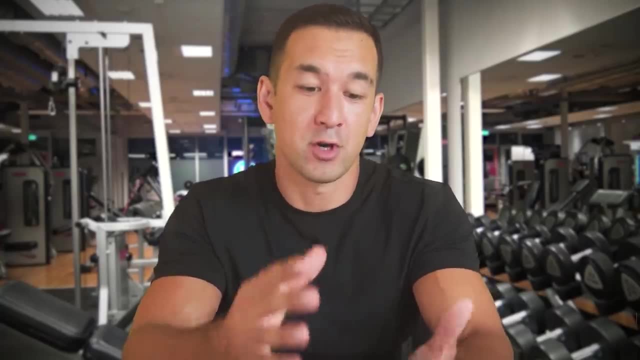 In reality, protein powder isn't even really a supplement. It's a lot more accurate to just think of it as a convenient food product. whether it's whey or egg or casein or pea protein, These powders are derived from whole foods. I mean, they literally are food. Little Miss Muffet sat on a 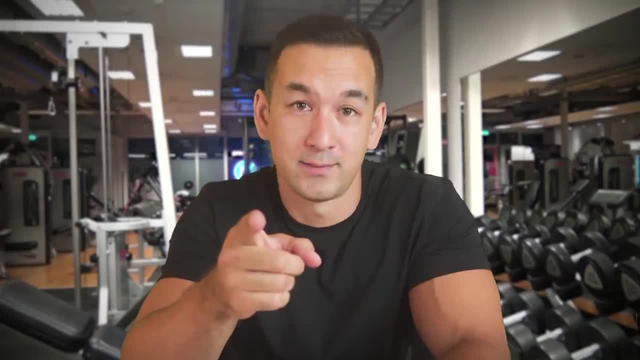 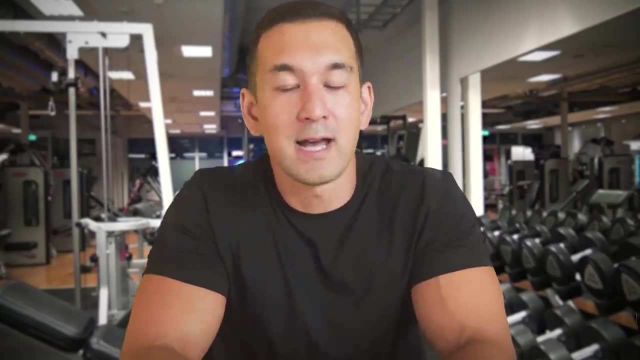 tuffet eating her curds and whey. She wasn't trying to make gains, She was just enjoying a meal. Or maybe she was trying to make gains. Look, I don't know. I wasn't there. I don't know what her specific goals were. 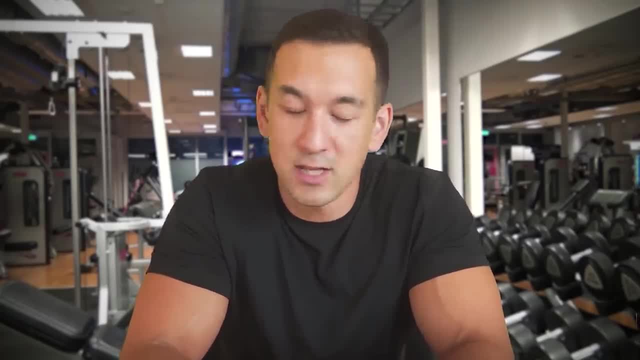 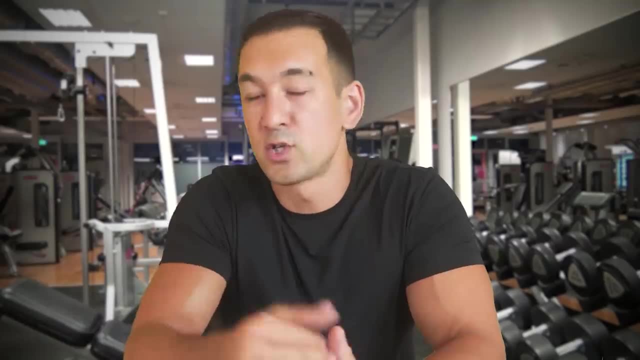 to be perfectly honest with you, I don't even know what a tuffet is. but that's not the point here. guys, We're going a little bit off track here. The point is: don't fall for the overhyped marketing. If you enjoy the taste and the convenience of a protein powder and you find 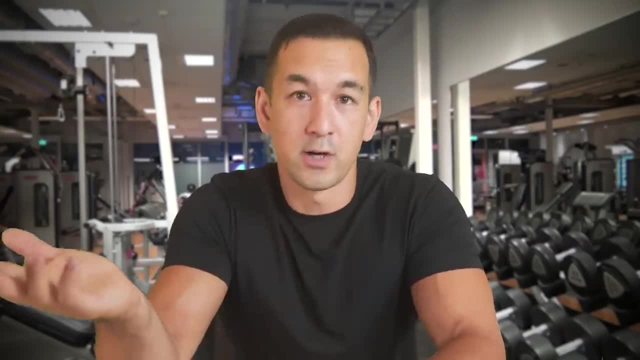 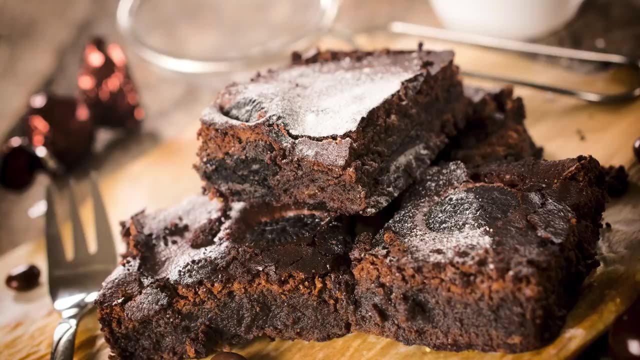 that it helps you hit your daily protein needs more easily, then go for it. I've consumed whey protein on a daily basis for 20 years now, whether it's in smoothies or yogurt or oatmeal- random high protein dessert style recipes. But if you'd rather just 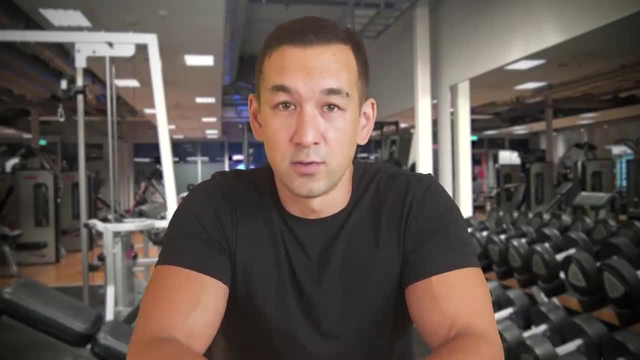 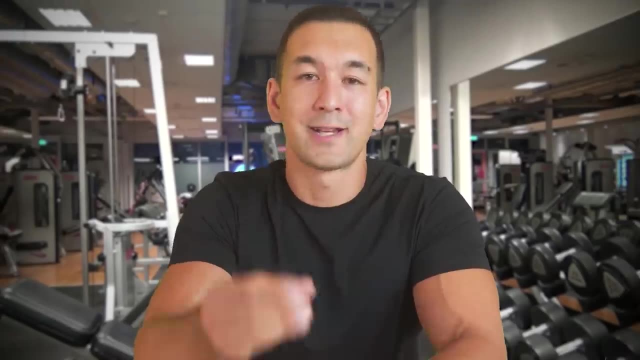 get all your protein from regular solid food sources, then that's fine too, And let me know in the comments what your personal preference is. I'd be genuinely curious to know how many of you are using a protein powder versus not. All right, And lastly, number three on the list. Now, this one isn't necessarily. 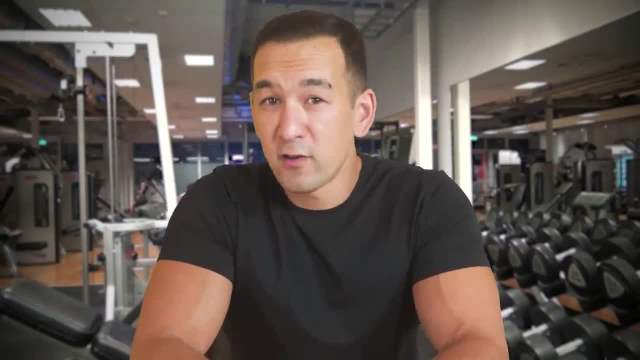 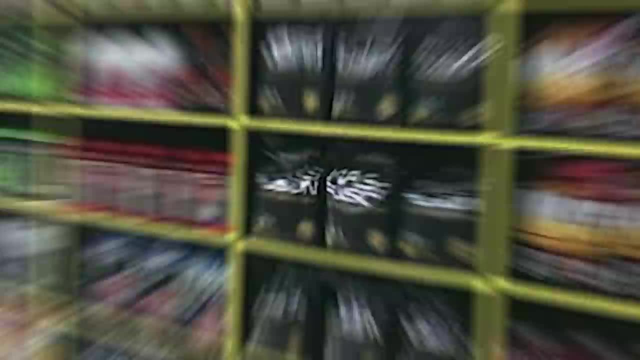 some sort of filthy scam, but it is something that you should be aware of, because it is something that a lot of supplement companies do take advantage of on purpose, and it can be misleading. It's something that almost every protein powder blend on the market does, and 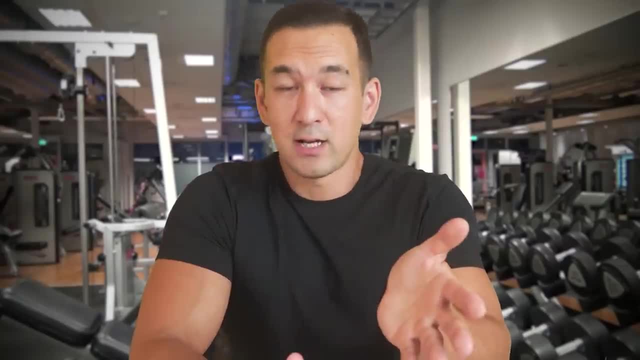 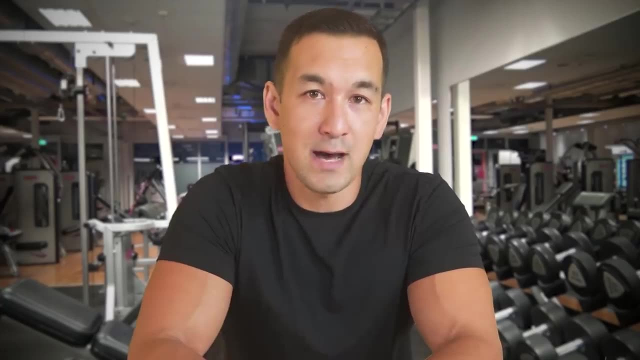 I honestly don't understand why this is so prevalent. What I'm talking about here is the use of proprietary blends when listing out the protein sources in the product. In other words, if you look at protein powders that include more than one type of protein, they virtually never tell you how much of each protein source you're getting. 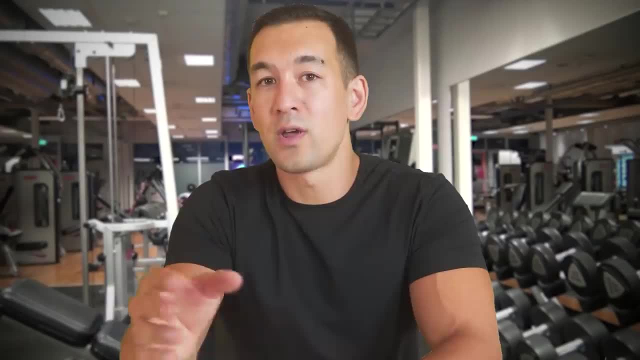 Instead, they'll just list off the total grams of protein, along with a list of the different types of protein that are in there, but not the specific amounts for each. The most common example. let's say you're buying a protein powder that uses a blend of whey concentrate and whey isolate. Almost never will the 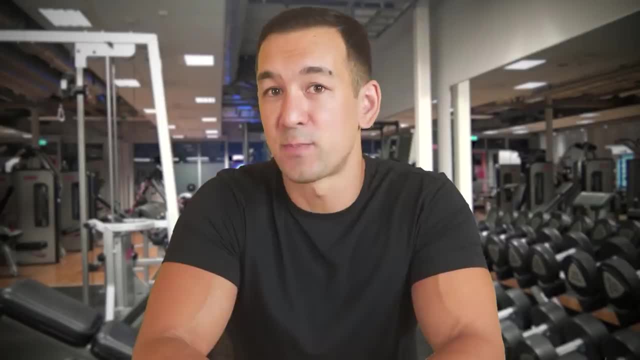 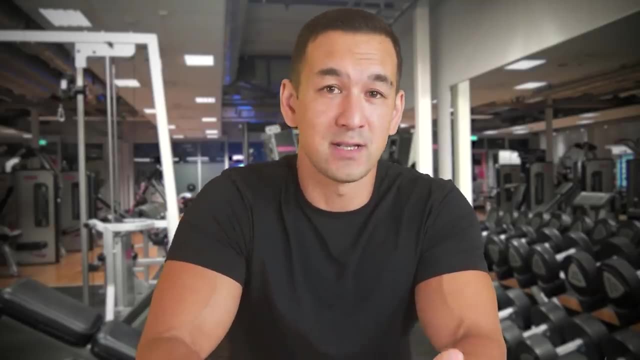 product state how much whey concentrate and how much whey isolate you're specifically getting, And instead it'll usually just be listed like this: Always keep in mind that the most prominent ingredient always has to be listed first, And so, for all you know, this could very well be. 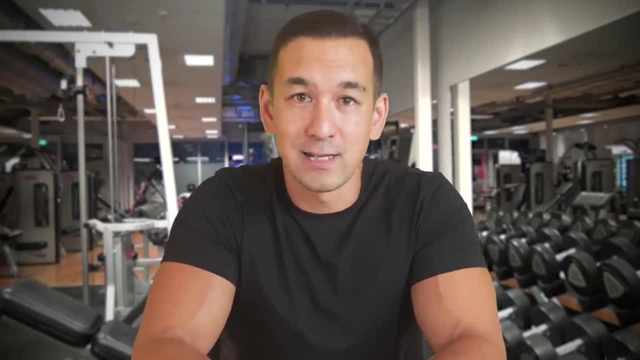 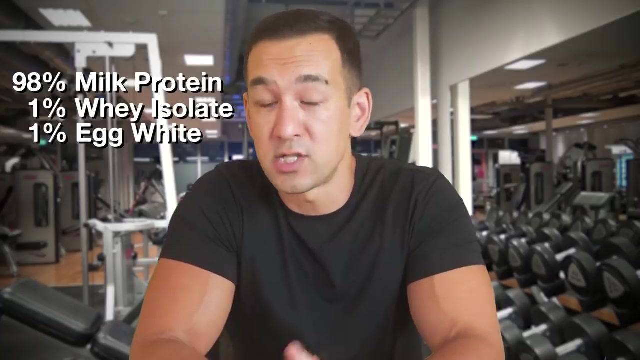 95% whey concentrate and 5% whey isolate. Or if you're buying a blend of, say, milk protein, whey protein isolate and egg white protein and it's using a proprietary blend, again it could literally be 98% milk protein, 1% whey isolate and 1% egg white protein. You just have. 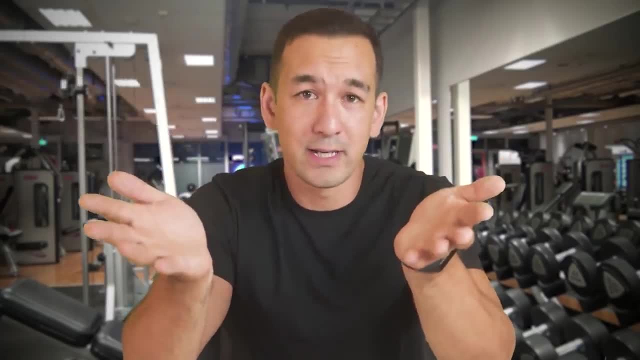 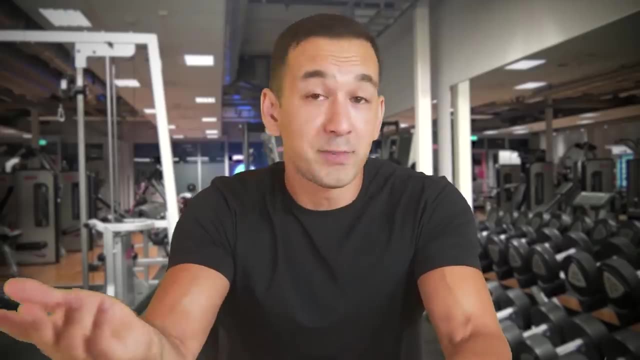 no way of knowing. Now, how much does this actually matter in a practical sense? Well, you know, if you're already using a certain protein blend and you're happy with the macros and the taste and the price, then ultimately that's totally fine And it's not going to affect. 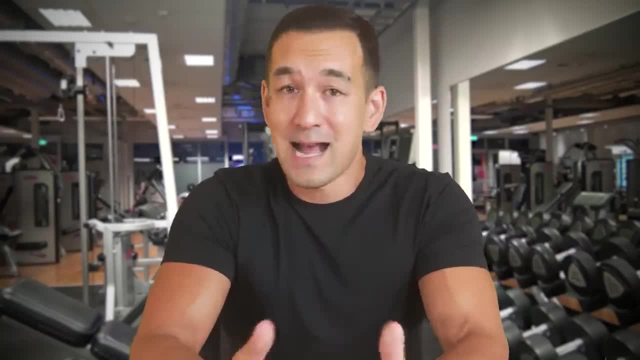 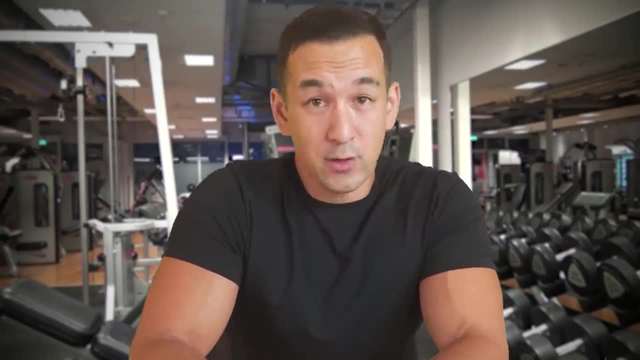 your actual muscle building results Because, like I said before, the exact type of protein you use doesn't really matter, as long as it's a high quality, complete source. However, what I would say is that if you're in the market for a new protein powder, then it is something to take into account. For example, if you were 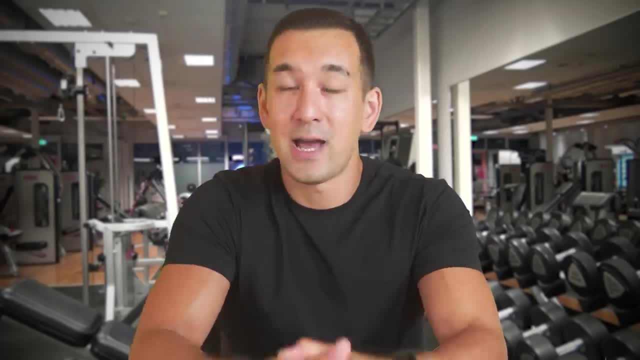 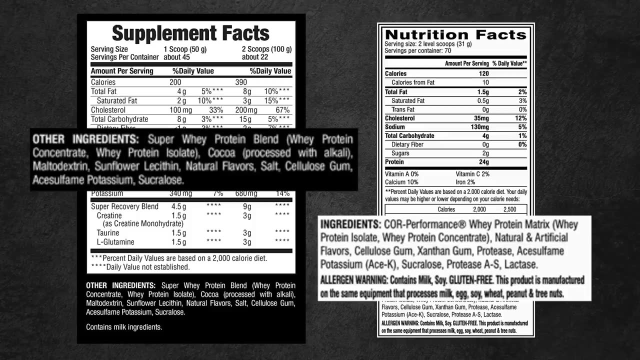 looking for a whey concentrate, whey isolate blend and you had, say, two different products. one lists whey concentrate first on the label and the other has whey isolate first and the price is comparable between the two, then you'd probably want to go with the one. 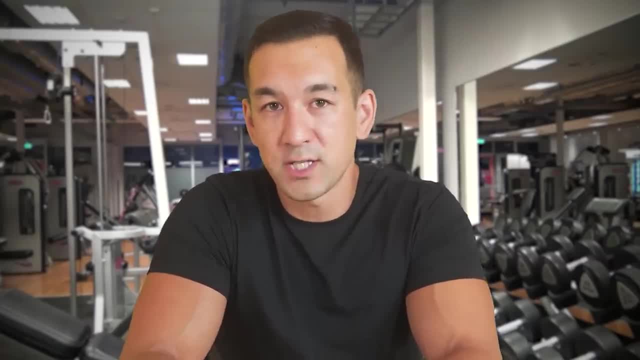 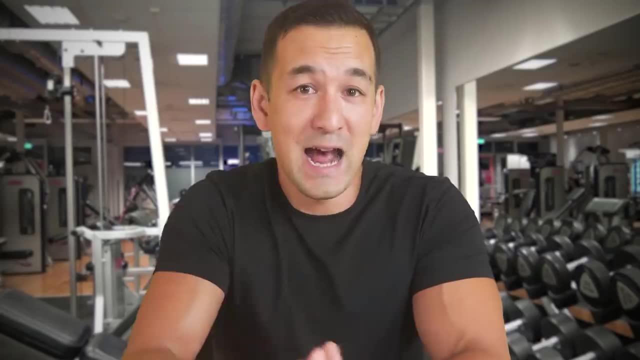 that lists the whey isolate first. You know there's nothing inherently wrong with whey concentrate, but it does tend to be a little bit heavier on the stomach, It doesn't mix quite as well And it does have a stronger sort of protein aftertaste to it. So by going with the one that 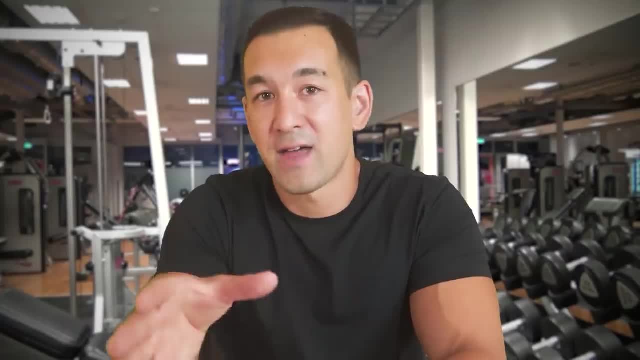 lists whey isolate first, then you'd probably want to go with the one that lists whey isolate first. You at least know that more than half of that blend is whey isolate, Whereas with the other products it could be almost all whey concentrate with just a tiny bit of isolate sprinkled in. 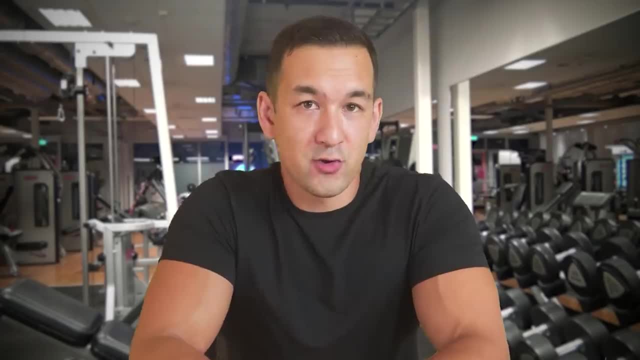 And the direct practical aspect aside, I just think it comes down to basic transparency and labeling, You know. I think you should know exactly what's in the supplements that you buy. Most of us don't accept pre-workouts that use proprietary blends, because we want to know. 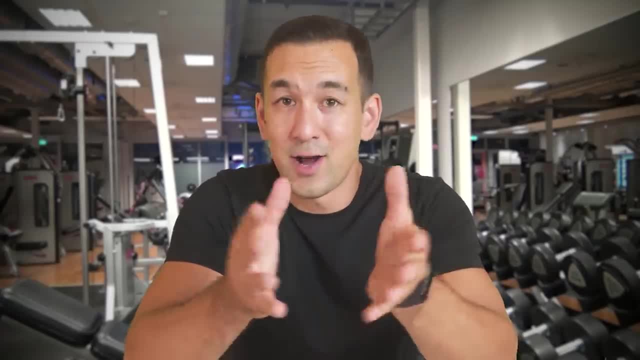 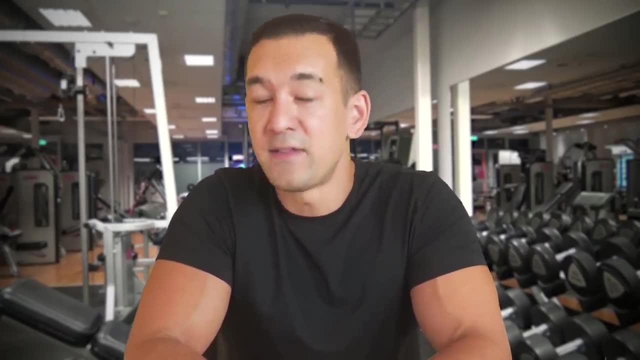 exactly how much of each ingredient we're getting, And while that's not directly comparable to protein powders, it is the same general idea And I think that if you're looking for a whey isolate, if companies are selling protein blends, then they should list off how much of each protein. 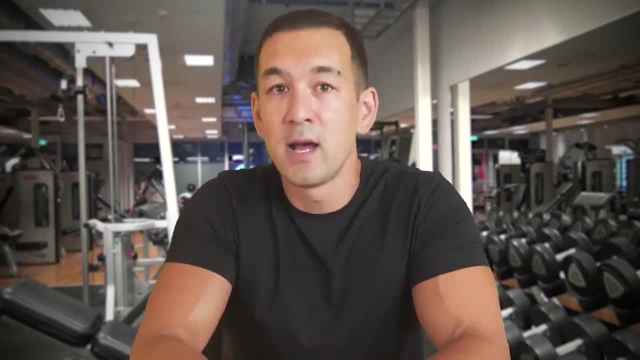 source is included, And Real Science Athletics, which is my own supplement line. like I said, we do have a protein powder in development right now which will be out in a few months, And with that product, you definitely will know exactly what you're getting in terms of the exact